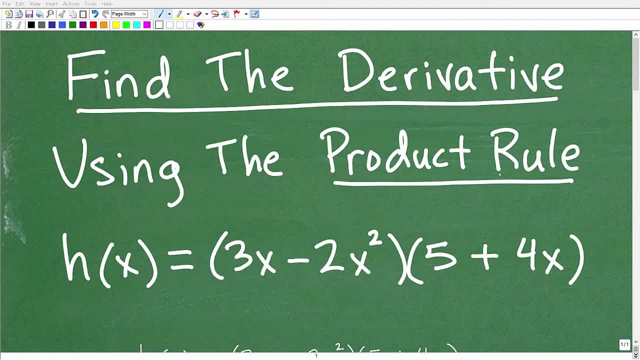 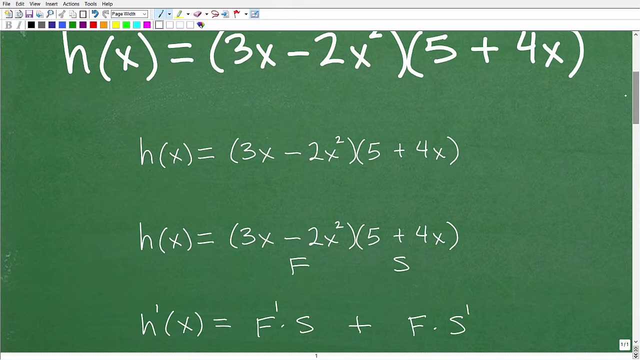 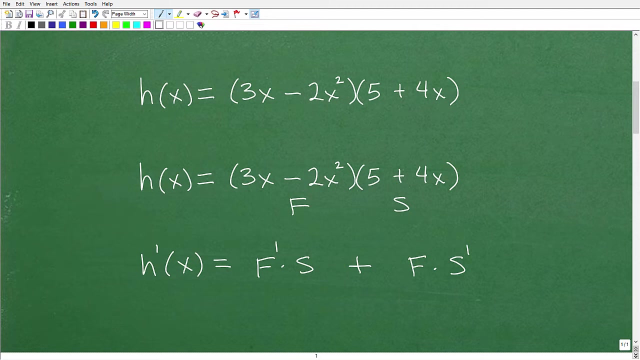 product rule, excuse me, is one of those just key fundamental rules that you're definitely going to have to commit to memory. So let's go ahead and find the derivative of this particular function. This is a pretty nice basic example to illustrate the product rule. Okay, so let's go ahead and just get this in a little bit clearer writing. I already pre wrote this out. So here is our function h of x, And first of all we're talking about the product rule. So product means what? 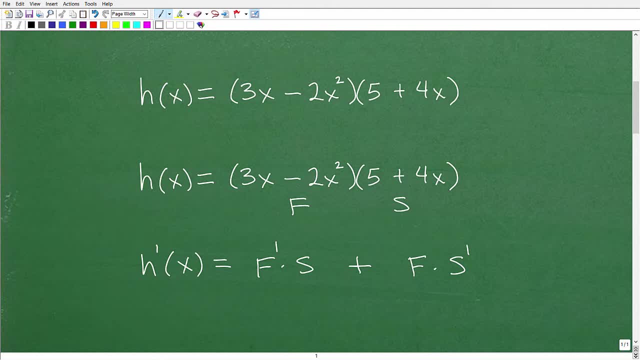 It means something being multiplied by something else. So if we look carefully here you can see we have one function. let me just write this here: we got one. not well, it's a function, but we have something being multiplied by something else. So we have a product. So when we're asked to find the derivative, first derivative h of prime of x, here, okay, and we have a product going on, bells should go off and be like: okay, product. 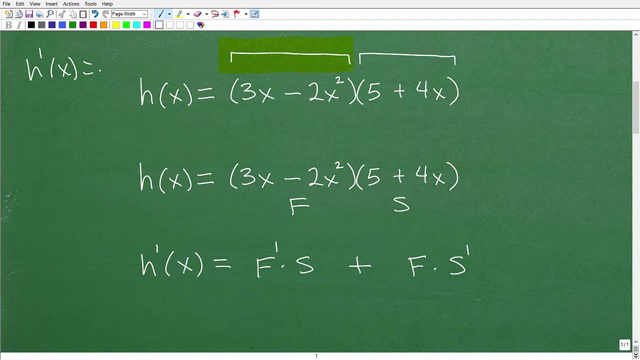 derivative. how about the product rule? Now, that would be an excellent approach to doing this problem. Now, another way you could approach this problem is if you simply forgot the product rule- is you could just find the product. you can go and do all this multiplication and then apply your knowledge of finding the derivative from there. So that's another route And you should know that approach as well. But you know there are times where you're going to just have to. 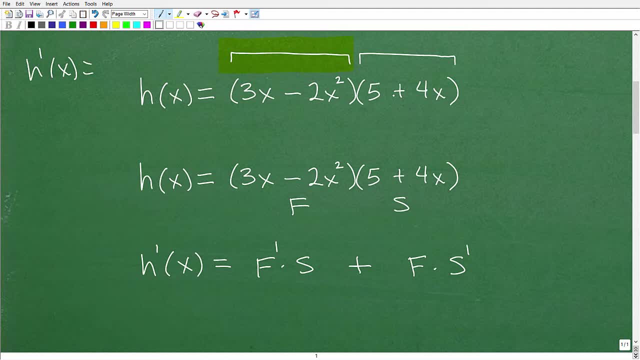 simply use the product rules. there's no other options. okay, especially like a trigonometric type of functions, etc. But the point of this video is just to illustrate the product rule and how to use it. Okay, so again. so we see that we have a product going on here And here we have. when we look at this product, let's just go ahead and identify the one of these terms. here is like the first function And here we just will identify this kind of 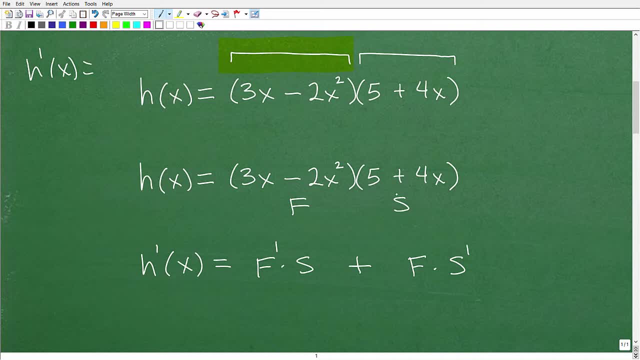 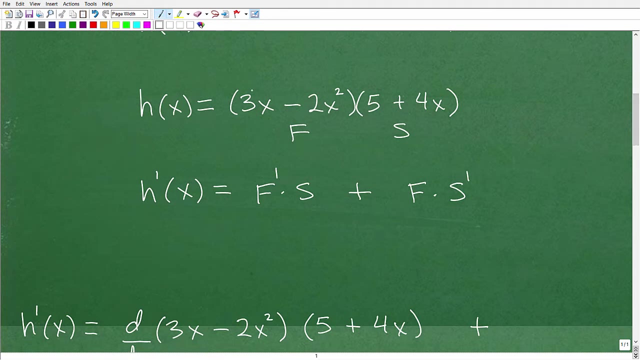 here is the second function, So f and s, and there's a number of different nomenclature that you can use, notation you can use to illustrate the product rule, but this is pretty straightforward, So let's just use this basic nomenclature here. So we have a function and it's made up of the first function times a second function, right, That's h of x. h of x is the product or is equal to the product of this first function times this second function. Okay, so the product rule is: 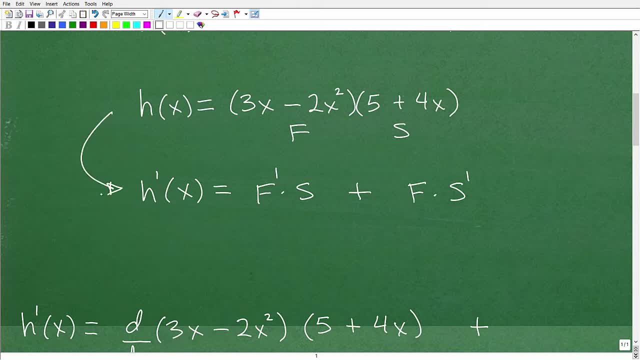 basically this: if I want to find the first derivative h prime of x, I can just follow this basic formula right here again stylistically and mathematic. but there's variations of mathematical notation, So in your notes, or your teacher might have given you the product rule a little bit differently than this, but it's still the same, believe me. So we have the first function times, a second function. So it's just going to write for first function times, section second function, plus first function times, second function. 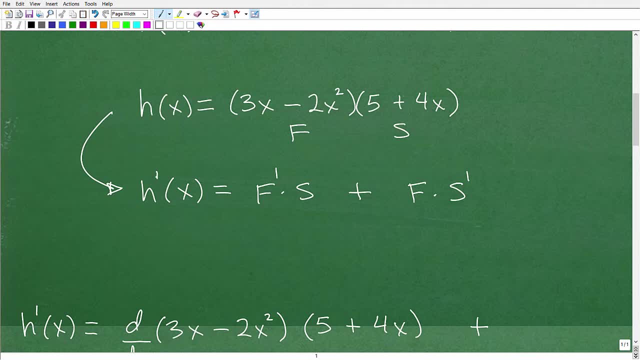 So the first derivative of this function h of x is going to be the first function, prime. So we're going to find the derivative of the first function, we're going to multiply by the second, then we're going to add it to the first function times, the derivative of the second function. So I like to kind of keep this notation nice and simple. So this is essentially the product rule. Okay, so if you can remember this, 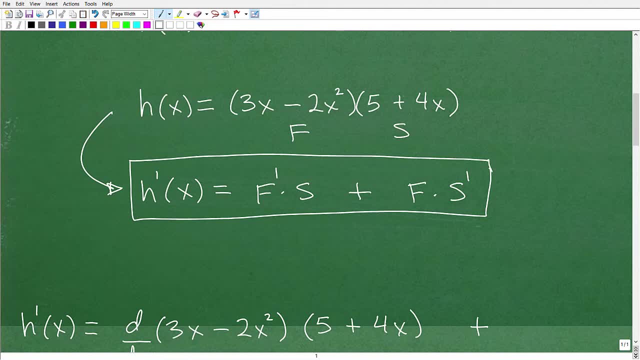 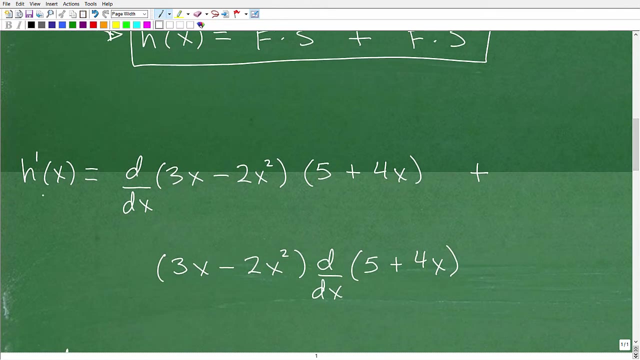 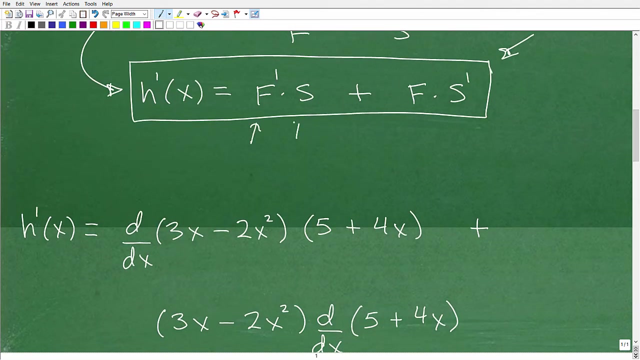 then you're going to be good to go anytime you're asked to find the derivative of a product. Okay, now let's get into the problem here And write the notation out. So let's keep this in mind. So this is going to be our h of x. Now, from our original function we're going to find the derivative of the first function. Okay, so I'm just kind of just follow along, I'm just going to kind of write this out and it's appropriate notation. So 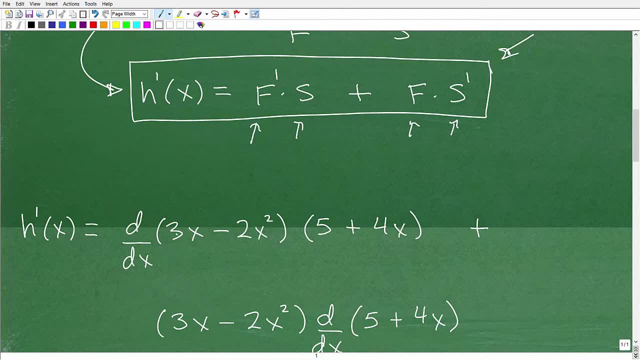 I'm going to find the first derivative, so d of x times. I'm sorry, I'm going to find the derivative of the first function, so I'm going to write it like so: okay, so this is the notation 3x minus 2x, squared very carefully, and I'm going to multiply by that second function. okay, I'm not taking a derivative of that second function. 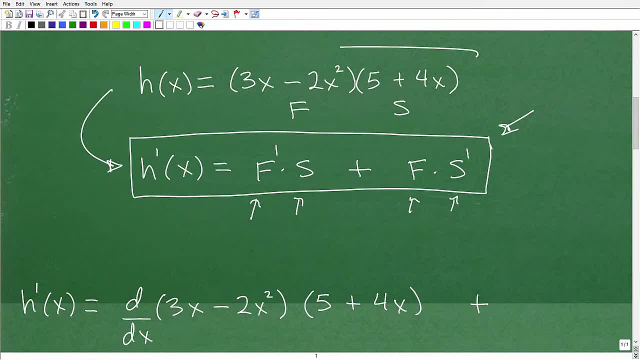 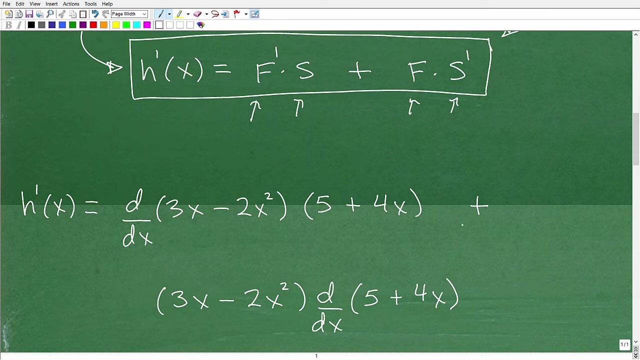 Now remember, here is our problem. so keep this in mind: big part of doing calculus is just keeping all your work nice and neat and organized and structured. so if you want to write this down to reference the video as we go along, okay, so this is the first function. that's the second function, all right, so I'm taking the derivative of the first function and multiplying by the second function. I'm going to add it to that first function and I'm going to multiply by the derivative of the second function. 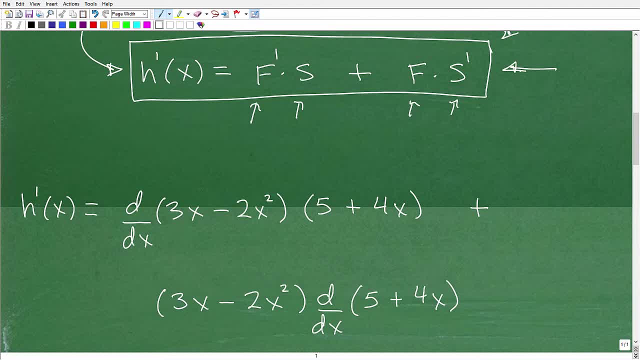 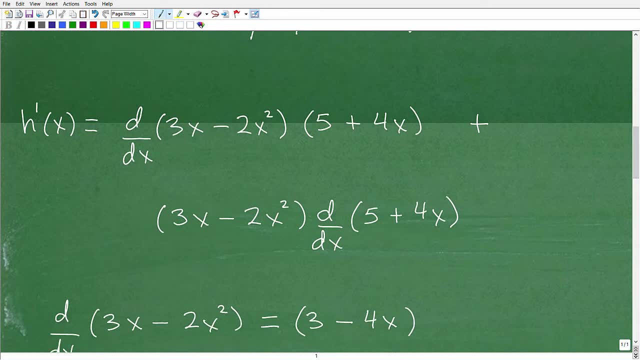 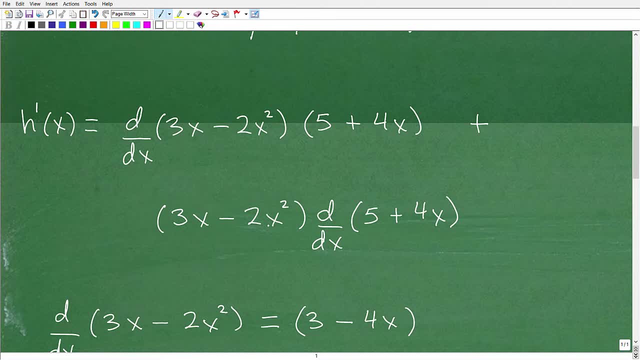 You know, if you didn't set it up correctly, then they would be like: oh, your answer is wrong because you don't even understand the product rule. But if you set up the product rule correctly and you happen to make a little error along the way, well, that's a little bit different. 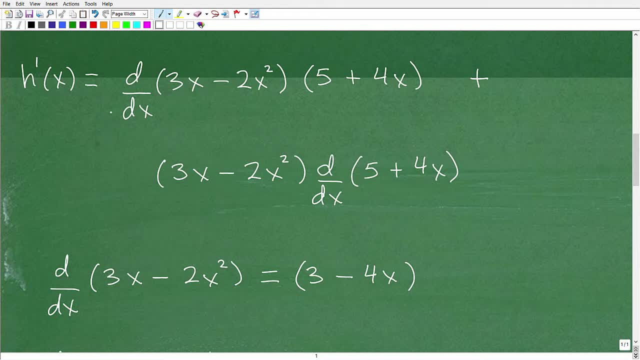 OK. so now we need to be able to make sure you understand how to find the derivative of a function like this and the derivative of function like this. So let's go ahead and find the derivative of each of these little functions and don't plug everything back in and simplify this. 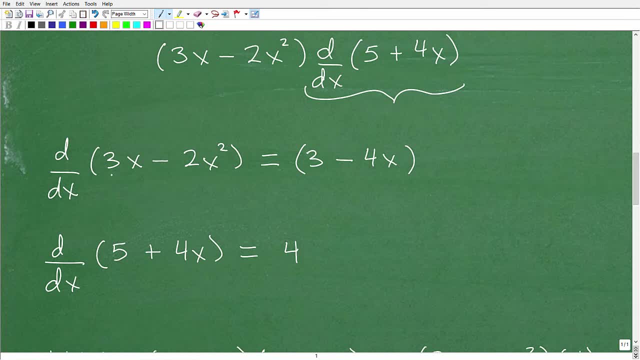 OK, so let's take this first one. So how do we find the derivative of 3x minus 2x squared? OK, so if we're using the product rule, you should already be able to find the derivative of polynomial functions like so: 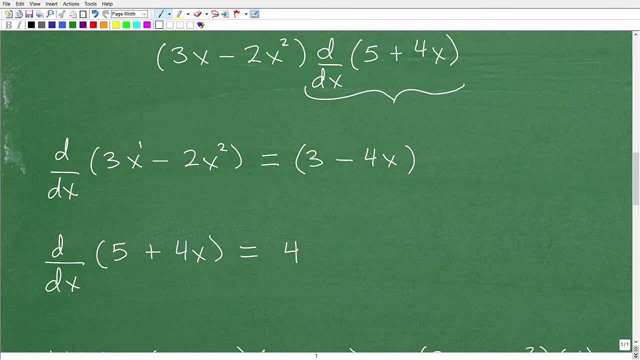 OK, so here's a little one. So the first derivative is going to be one times three. OK, so that's going to be three. And then we're going to drop this down by power, So that's going to be one minus one or zero. So it's just going to be three. 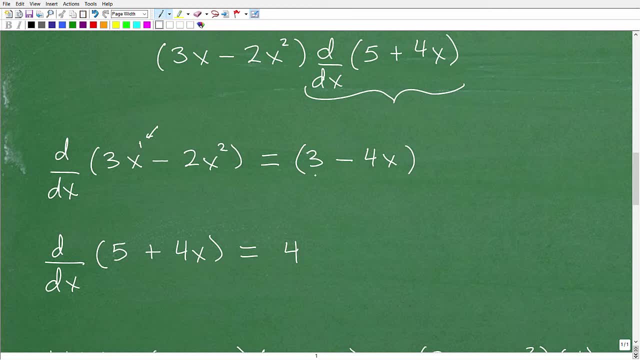 OK now. Now, if you're lost at this point in the video in terms of not knowing how this derivative equals this, then you might want to look at some other videos, because the product rule is kind of a little bit further along in terms of finding the derivative. 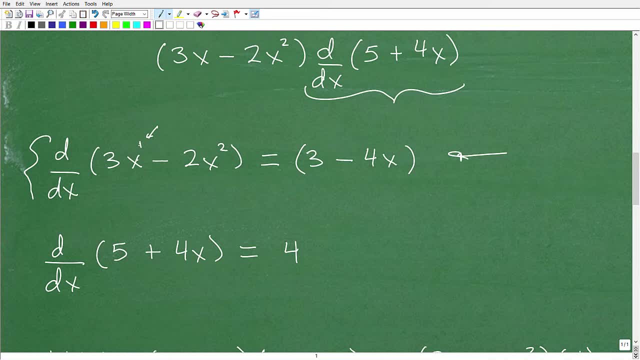 OK, but let's continue on here. So it's going to be one times three, times x. Then we're going to drop this down to x, to the zero power which is one. So that's three. Now here, this is going to be two, this little exponent, or two times negative. 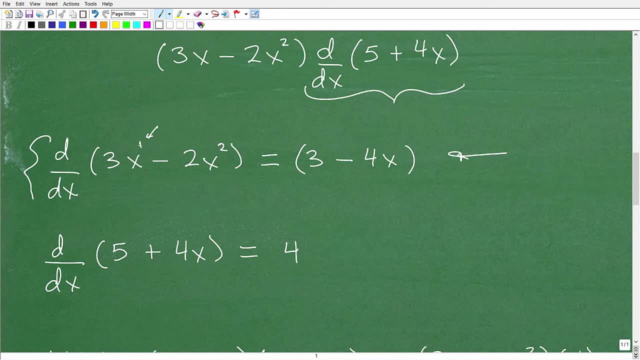 Two is going to be negative four, Then it's going to be x, or drop this down by one, So that's going to be x to the first, All right. So if you know that the derivative of this is equal to this, then you're good to go. 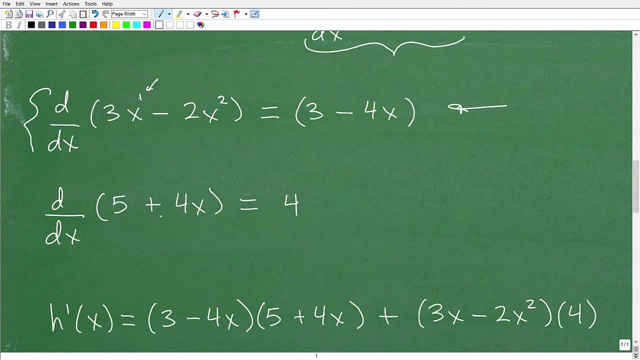 All right. So let's go ahead and find the derivative of five plus four x, And then here the derivative of a constant is zero. And then here we have this little one. So one times four is just going to be four, And I'm going to have this as x to one minus one to zero. 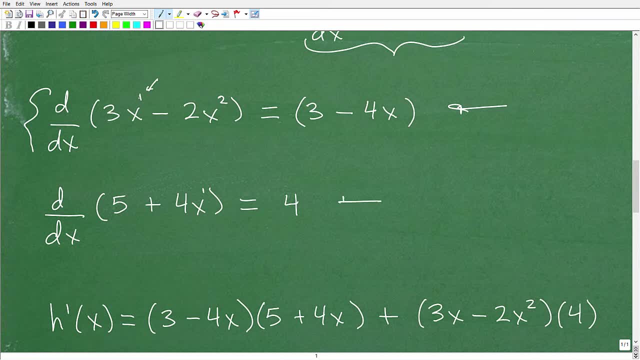 So this is just going to be four. All right Now, I didn't mean to kind of blast through finding the derivative of these particular functions here. But this video- you know it's focus- is using the product rule. This is more of a different type of video in terms of finding derivatives of basic functions, polynomial functions, etc. 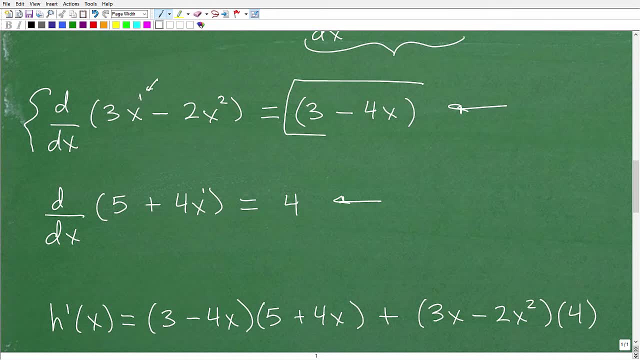 All right. So if you're good to go and you understand that the derivative this is that and the derivative of this is this, then we could just simply go ahead and plug everything back in. OK, so let's go back up here to when we set things up. 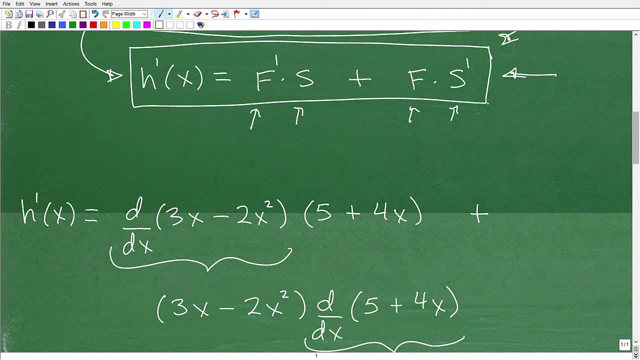 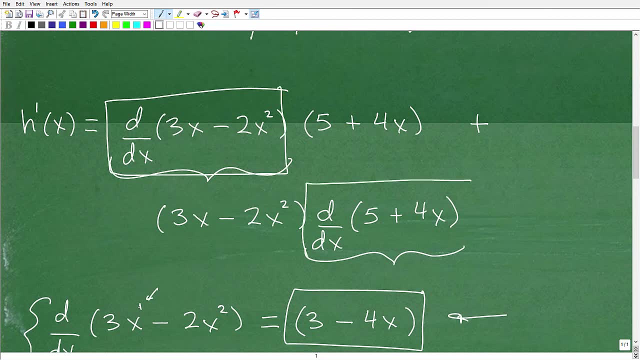 OK, so this is the formula that we set up for the product rule. OK, so what we just did is we found the derivative of this and we found the derivative of that, And now we're just going to plug in what we just found right into this formula. 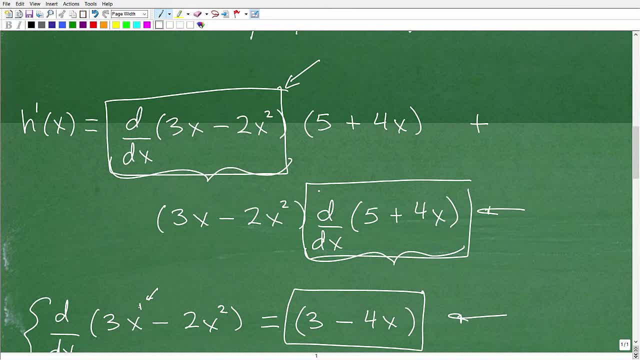 Do you want to write all this down? So I'm not kind of going back and forth in the video too much to confuse you. Then that would be OK. All right, So we're going to substitute this, The derivative, for three x minus two x squared, All right? 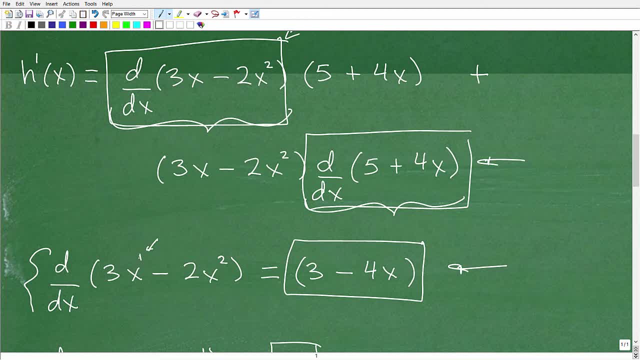 We found as three minus four x, and the derivative of five plus four x we found as four. So we're going to substitute those values in here and just kind of plug all this in into this function here. Let's go ahead and do that. 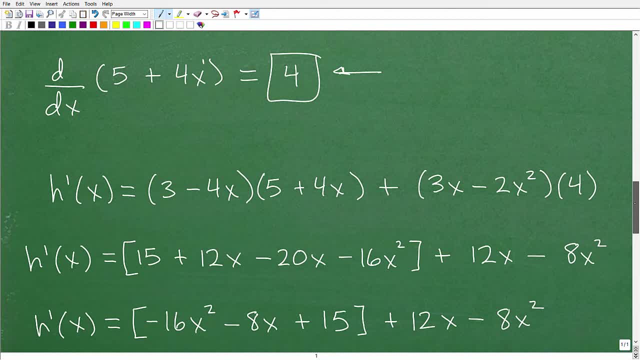 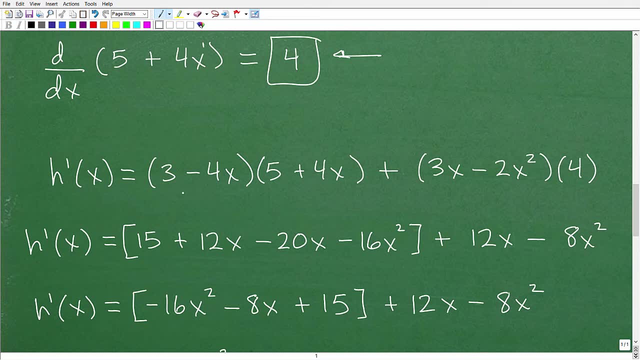 Now, And we do when we do that, we get H prime x equals three minus four x, which again is the derivative of that first function times the second plus that first function times the derivative of the second function. All right, So here is the product rule, all kind of mostly simplified Right. 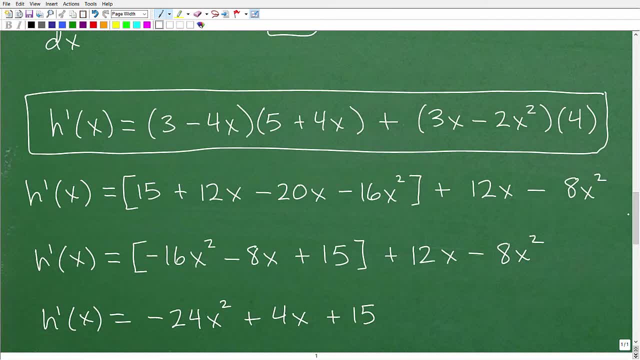 So at this point, for to get the final answer, we just got to go ahead and apply our handy dandy algebra Skills And we're going to multiply these guys together. multiply this together and simplify, Right. So be careful, because calculus students tend to make a lot of algebraic errors. 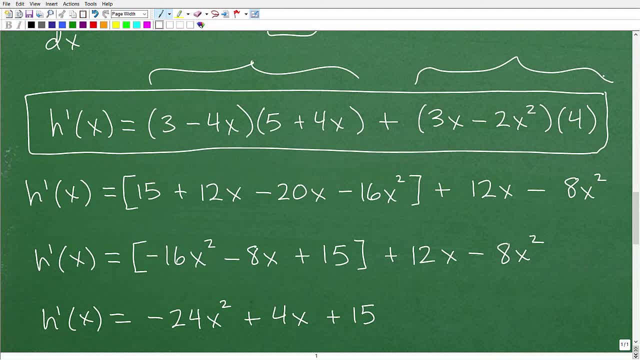 It's just normal. So when you're doing calculus, not only do you have to keep all these concepts of what you're learning about calculus of mind, you really have to be very careful with the algebra, because just because you're in calculus doesn't mean you're somehow- you know- above and beyond. 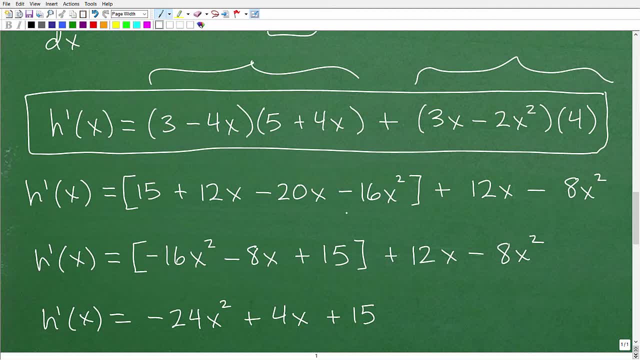 So you're making these little algebraic errors. It's very, very common, I would say. oh, in my experience maybe, like maybe 50 percent of the time, if you make an error, it's probably not because you don't understand the calculus. 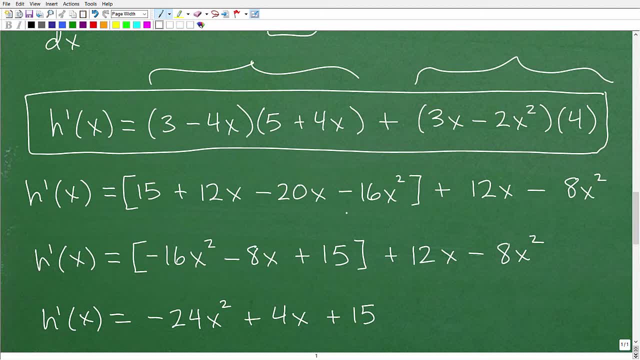 It's because you're making some little arithmetic mistake. you know something that you would do in algebra one, algebra two, student level. OK, All right, So let's go ahead and just multiply these two things together, these two binomials. 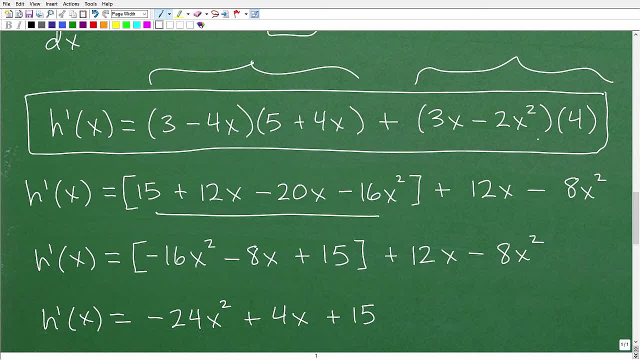 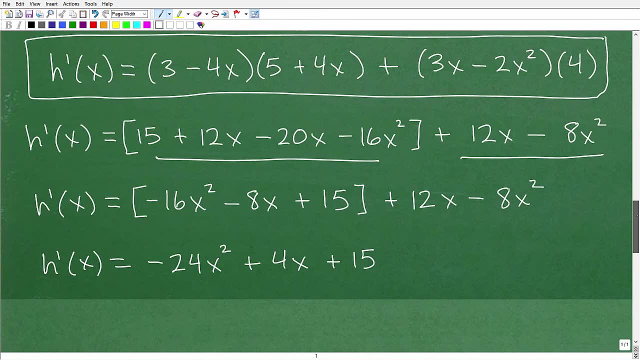 And you get this and we're keeping things in brackets and then we'll do the distributive property. here We get this. You can kind of follow along, Do the math yourself if you like, And of course I'm just simplifying along the way. 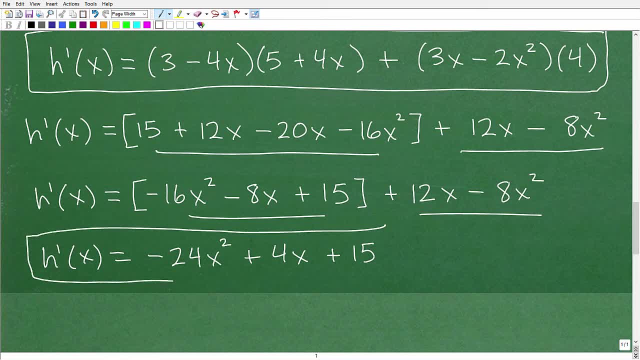 And when we finally get done, we get H prime, the first derivative of that function, which was a product. Remember the regular? the original H of X function was a product. And here we have the first derivative of that function And here it is right in its glory. 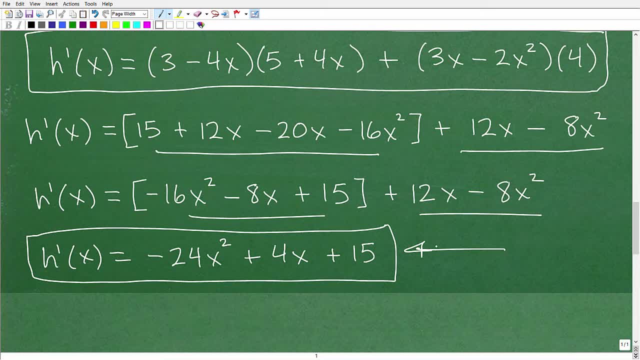 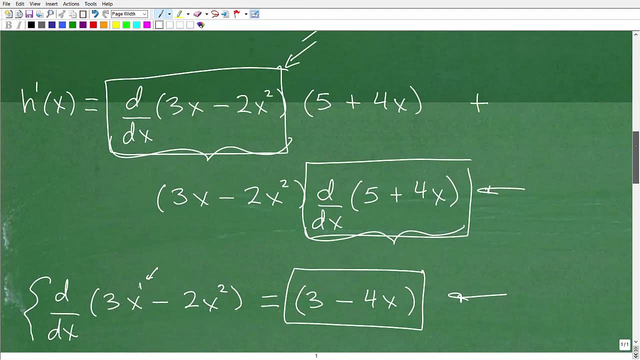 Negative: twenty four X squared plus four X plus 15.. OK, so that is the answer. Now again, you could have taken the approach: Let's go way back up here. You could have said: OK, you know what? I don't want to deal with the product rule. 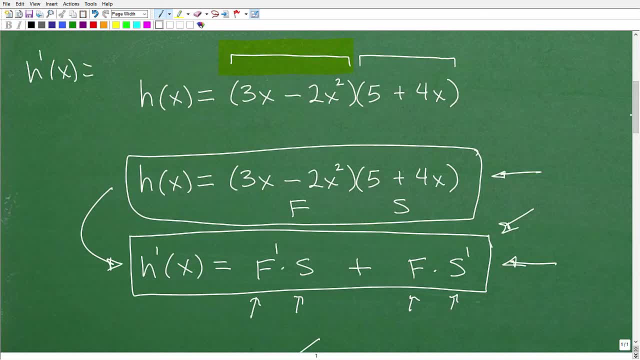 I forgot the product rule. It's just too confusing for me right now. So you couldn't just multiply these two together and have this one big function and then went ahead and found the derivative. that way, And that's equivalent as well, You would have gotten the same answer. 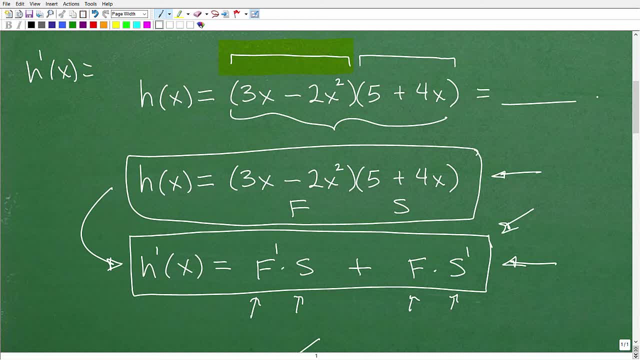 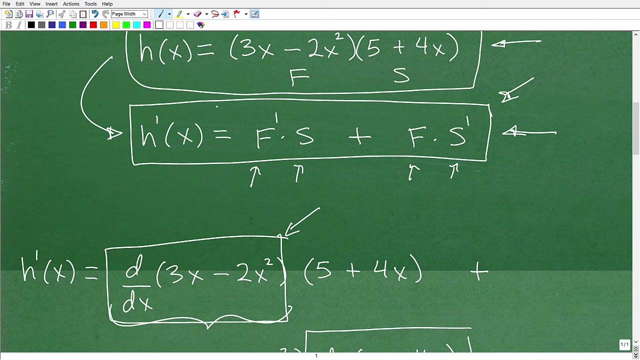 But you need to know the product rule in calculus is no way Again. we're around it. So hopefully this is a fairly basic example to you know. illustrate finding derivatives using the product rule. Now, one thing I can suggest to you, it's one thing that would work for me and it might work for you, is all these rules here. 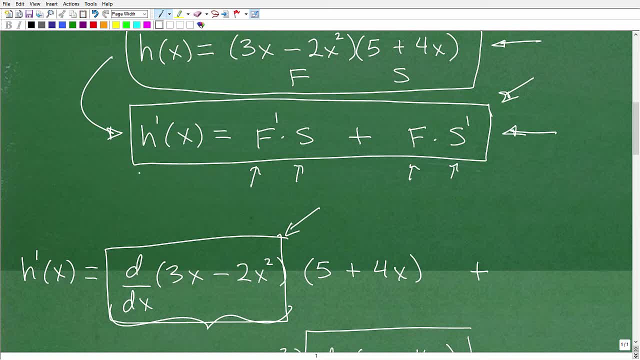 OK, you're, you know, depending on how your notes or your textbook or your teachers writing them, try to find a little bit simpler way to illustrate These rules. OK, so maybe instead of using function notation like here, like F of X times G of X plus, let's say F of X times G of X. 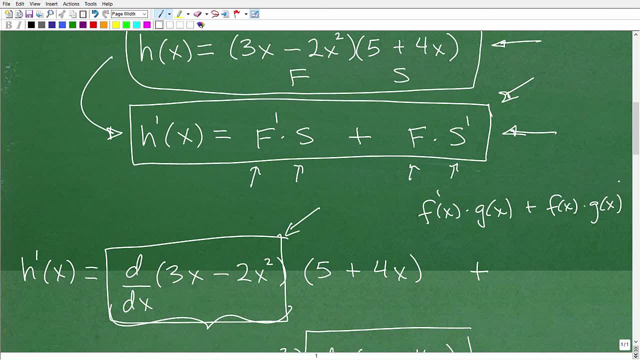 And then we'll have prime, and then prime like so. OK, so just try to find ways to simplify these formulas and maybe put like: first function, second function. come up with little mnemonics, little tricks, As long as you understand how to apply these rules. 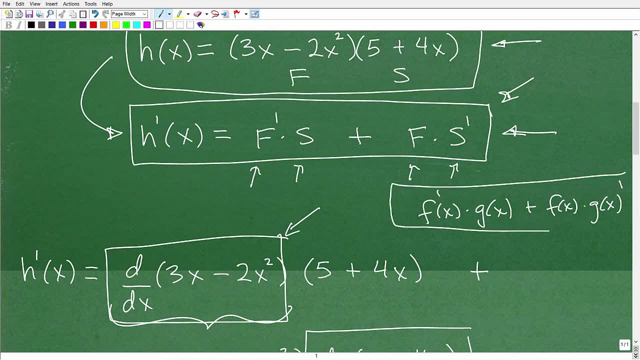 OK, you'll be OK. All right, To save you. you know a lot of writing in your notes, But you know, take notes that make sense for you. All right, Of course you got to make sure that they're mathematically correct. 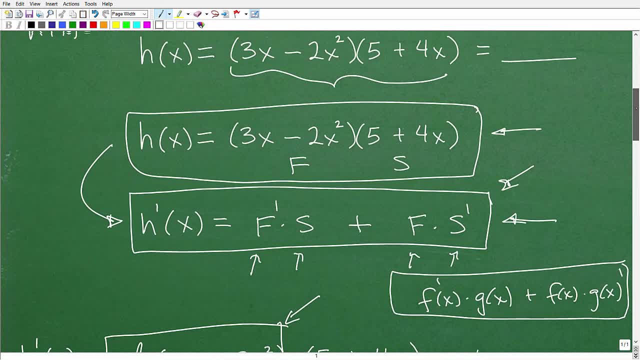 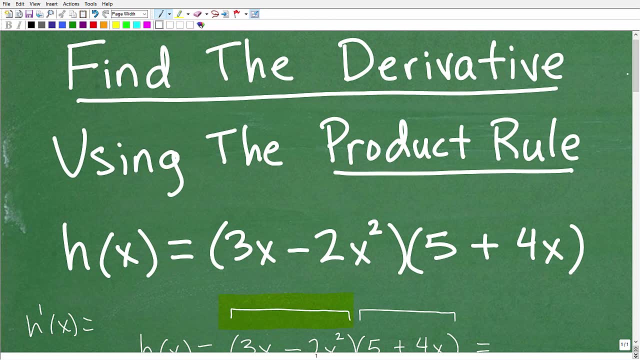 But you know, in calculus there's tons and tons of rules, derivative rules, integration rules, et cetera, et cetera. OK, so, anyways, hopefully I earned a thumbs up If I didn't listen. leave me some feedback either way.